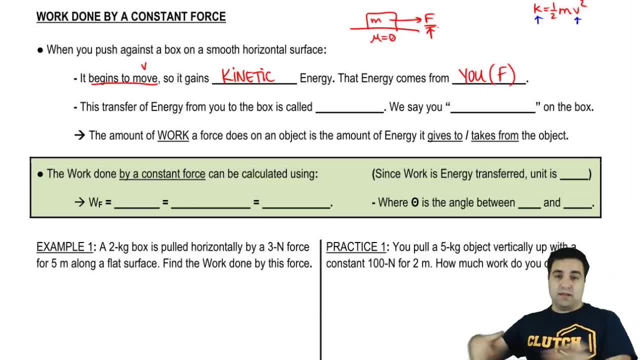 energy comes from you. You ate some food and the energy ultimately comes from the sun. right, The sun gives energy to the plant, The cow eats the plant and you eat the cow and then you push this box right. Very simplistic, but that's basically the idea: This transfer of energy you transferred. 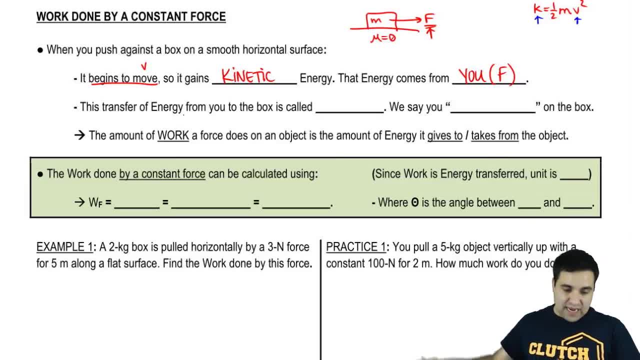 your stored energy into the box, into the form of kinetic energy. This transfer of energy from you to the box is called work. okay, So in physics that's what work means, And we see that in the physics of physics. We see that in the physics of physics, We see: 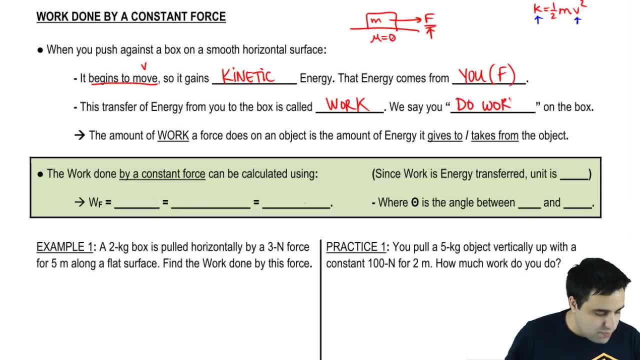 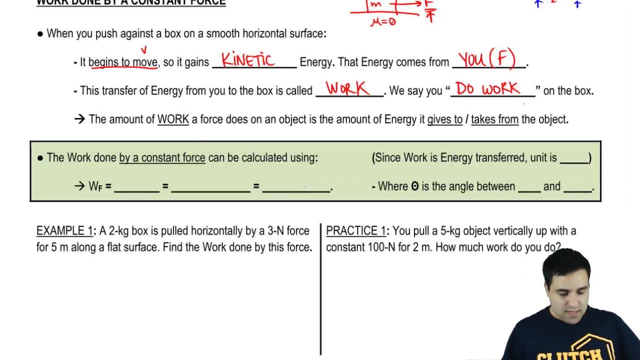 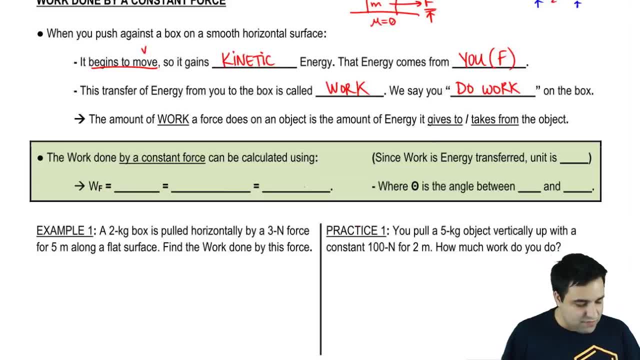 The amount of work that a force does on an object is the amount of energy that it gives to that object or takes away from that object. So if you push a box and you make it faster, you're giving it energy and therefore we're going to say we'll talk more about this later. 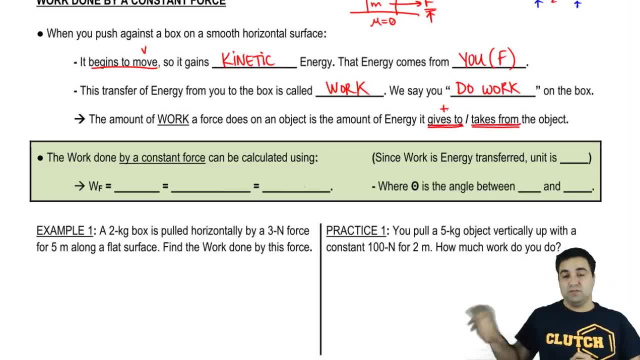 but we're going to say that you do positive work. If a box is moving and you push on it so that it slows down, you're stealing kinetic energy from that box. so you're taking energy away from the box. so you do negative work. 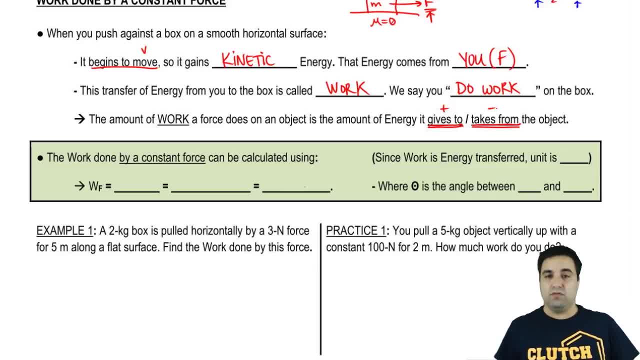 We'll talk more about positive and negative work later, but I want you to understand that the idea of work is that work is energy in transfer. It's you transferring energy? okay, To calculate work, the equation for the work done by a constant force. this only works. 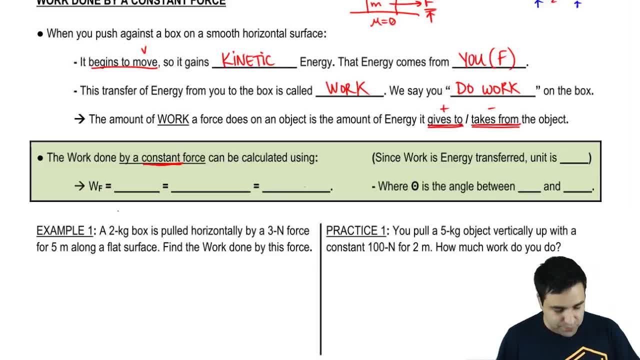 for constant forces can be calculated using this equation. okay, I'm going to give you sort of the fancy definition and then the useful one. So it's force which is a vector: the magnitude of force times the magnitude of displacement. 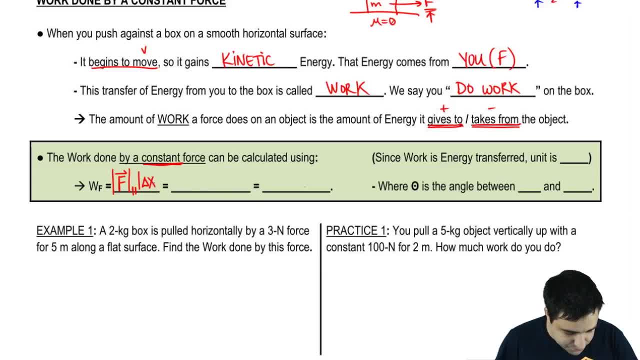 but these guys are supposed to be parallel to each other, okay, So that means that they're supposed to be parallel to each other, And the other lesson that I want to give you is that you have to be able to calculate this equation, Okay. 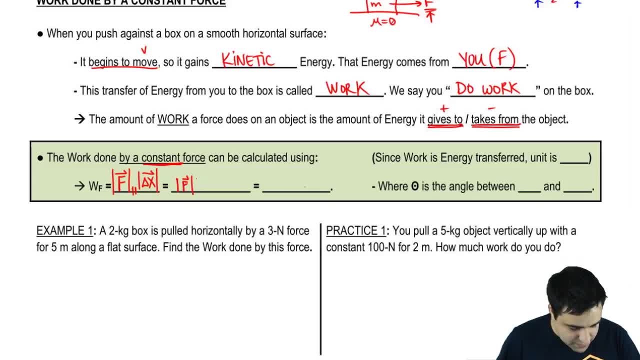 So the most fancy version of this would be F- delta X cosine of theta. If they're not parallel to each other, then you would do this: F- delta X, cosine of theta. where theta- I'll write this here in a second- where theta is. 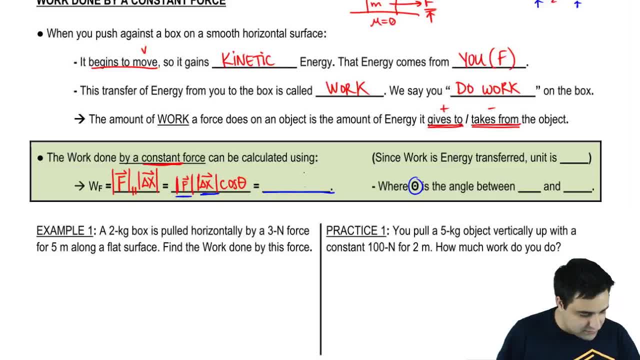 the angle between F and delta X. F and delta X- These two are vectors, so you can draw two little arrows and then it's just the angle between them. One way that I like to write this equation is I put a little arrow here to remind me. 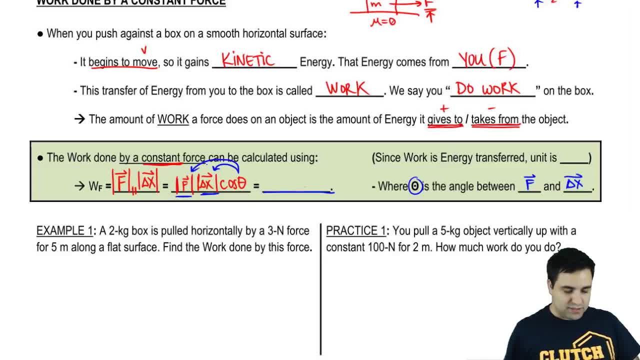 that theta is the angle between the two guys that are in the equation hanging out next to theta. Now, this is a lot of lines and arrows everywhere, so the simplest, the simpler version of this would be: F D, cosine of theta. okay, Now, that being said, remember this was originally absolute value. so when you plug these make. 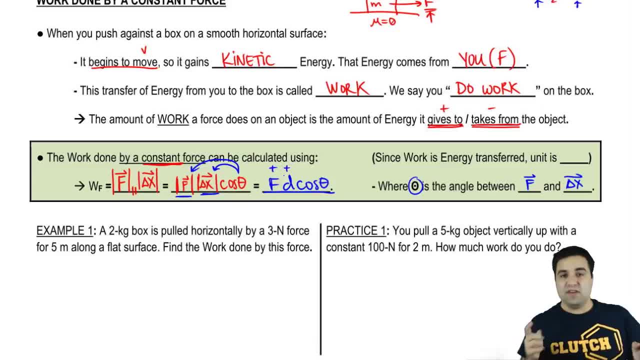 sure that F is positive and D is positive. okay, Even if you're moving to the left or if the force is to the left, it doesn't matter. okay, These guys will always be positive and this is the angle, cool. Now, last point here is: since work is energy transferred, work is just transfer of energy. 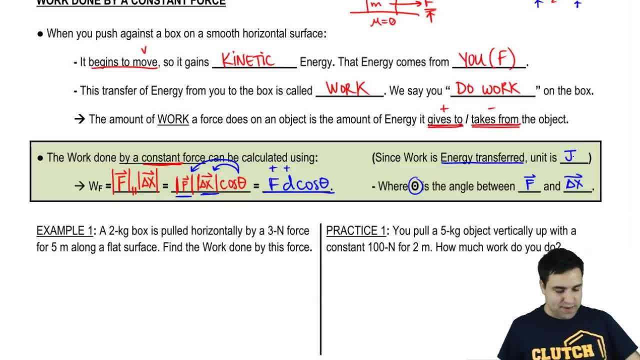 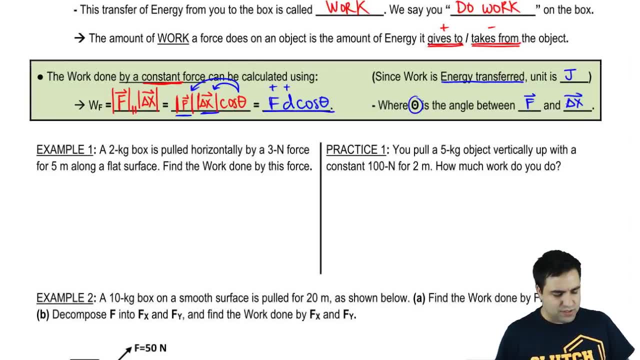 the unit of work is the same as the unit of energy joules. okay, Let's do some problems real quick. I'll do one and I want you guys to do one. So a two kilogram box is pulled horizontally by a three Newton force. 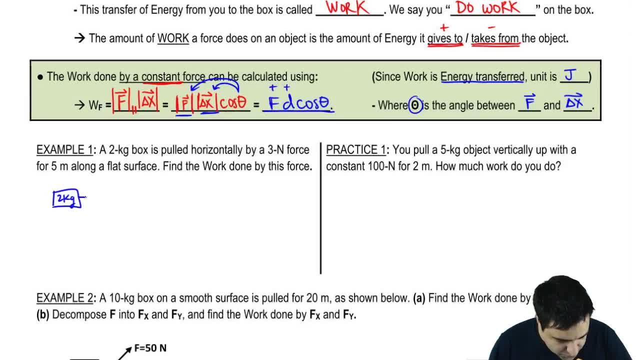 Let's do that real quick. Two kilogram box. It's pulled horizontally by a force of three, three Newtons for five meters. That's my distance. So I did this for a distance of five meters. So the idea is I pull and then, once the box has covered five meters, I just let it go. 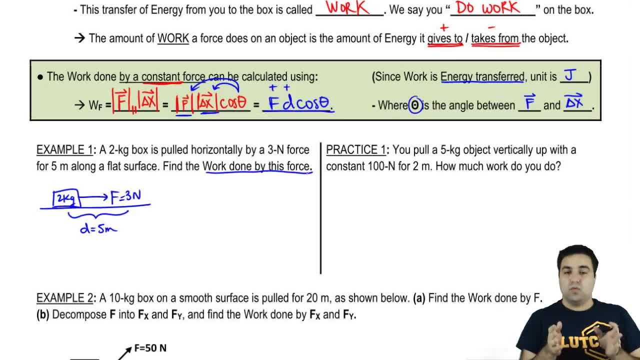 right. I want to know what is the work done by this force? okay, So works are done by forces, The work done by a force. F is right here, F, D, D, cosine of theta. okay, Now, F and D are pretty straightforward. 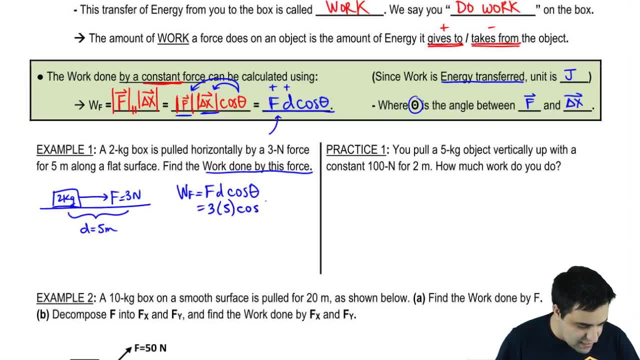 The force is three, D is five, But every time you get to theta, I need you to slow down and take it easy here and be careful, because there's some questions that are going to be tricky. Remember, it's the angle between these two guys. 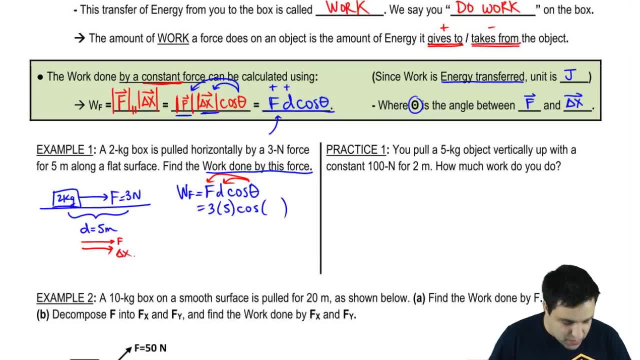 Force is this way, Displacement is this way. Notice how they're parallel to each other. They go in the same direction. The angle when two things are parallel to each other is Zero degrees. So this is cosine of zero And the cosine of zero. you plug into the calculator and you see that it's one.